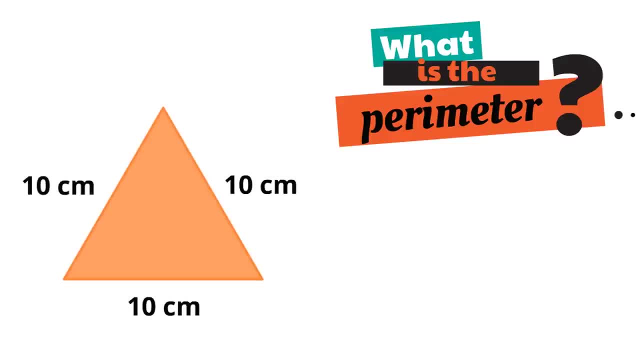 Let's pretend we measured it and each side is 10 centimeters. Now remember, to find the perimeter of a shape, we need to know the distance around the whole shape. So we just add the sides together, Plus 10,, plus 10,, plus 10.. 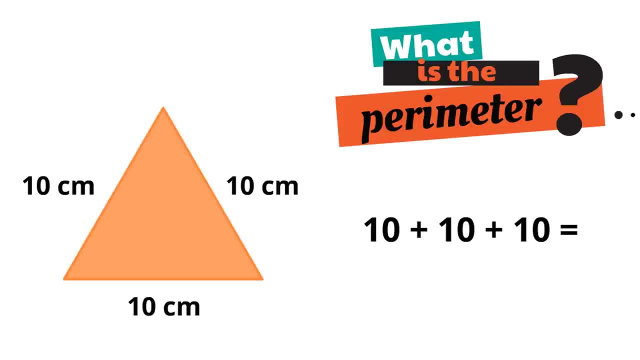 That's three 10s. What does that equal? Yeah, 30.. Awesome. The perimeter of this triangle is 30 centimeters. Remember, CM is an abbreviation for centimeters. 30 centimeters is the perimeter of this triangle. 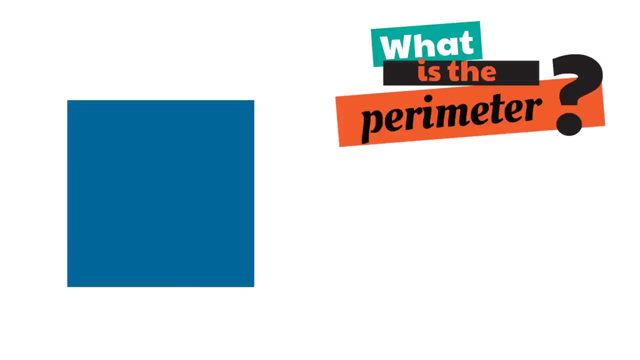 Okay, let's try this one. What is the perimeter of this square? First, we need to know how long all the sides of the square are. Then we can figure out the perimeter of the square. Okay, so this is a square. 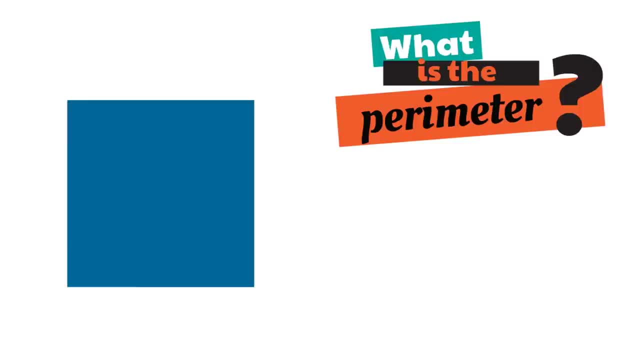 It has four sides and all four sides are the same size. Let's pretend we measured it and each side is one yard. Remember, YD is an abbreviation. YD is an abbreviation for the distance of a yard. Each side is one yard. 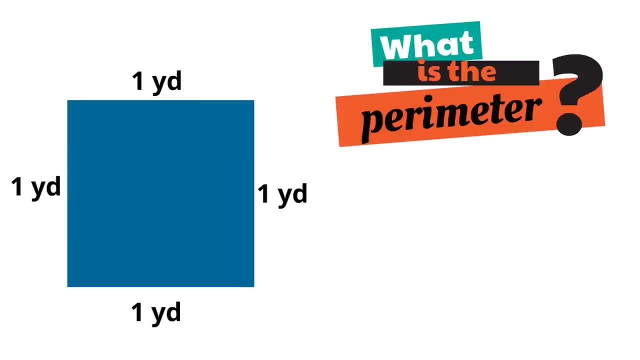 Remember, the perimeter is the distance around a shape, So we'll need to add all of these sides up. Okay, what's one plus one? plus one plus one, Yeah four. The perimeter of this square is four yards. 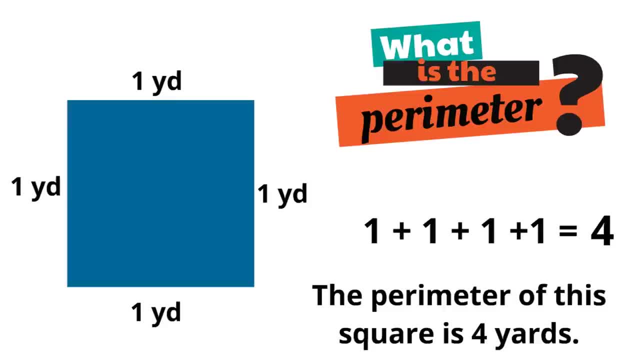 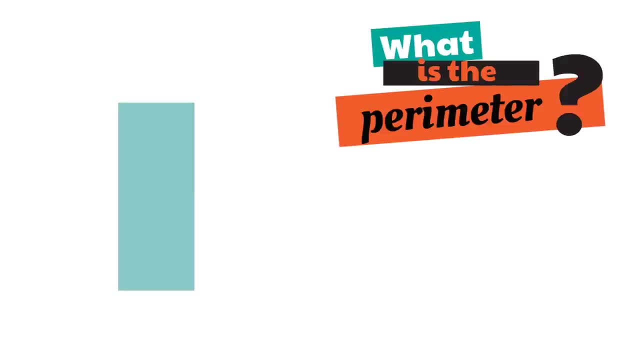 The perimeter, remember, is the distance around a shape. If you were to go around this entire square, it would be four yards. Okay, this is the final one. What is the perimeter of this rectangle? Well, first we need to know how long all the sides of the rectangle are. 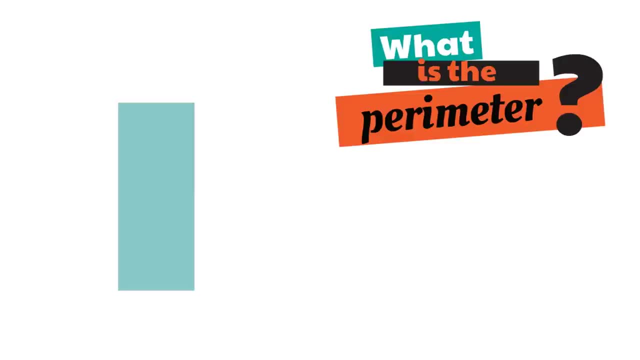 Then we can figure out the perimeter. Remember, a rectangle has four sides and two of the sides are shorter than the other two sides. With this rectangle, let's pretend we measured it at one meter on the short sides and three meters on the longer sides. 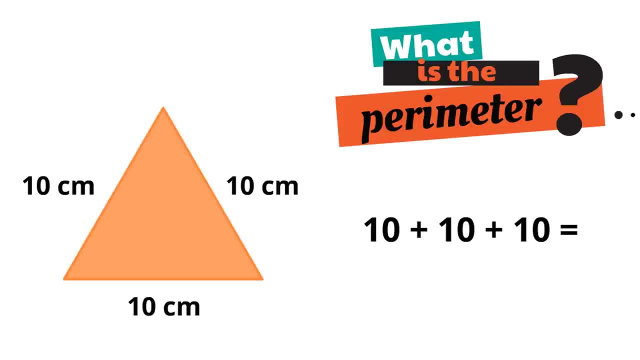 That's three 10s. What does that equal? Yeah, 30.. Awesome. The perimeter of this triangle is 30 centimeters. Remember, CM is an abbreviation for centimeters. 30 centimeters is the perimeter of this triangle. 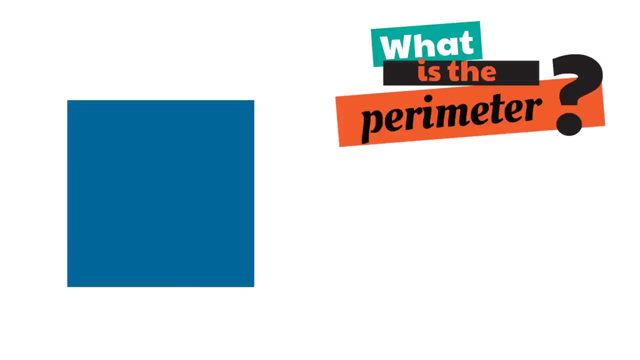 Okay, let's try this one. What is the perimeter of this square? First, we need to know how long all the sides of the square are. Then we can figure out the perimeter of the square. Okay, so this is a square. 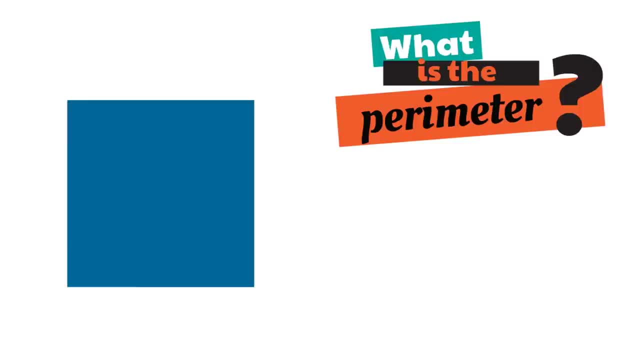 It has four sides and all four sides are the same size. Let's pretend we measured it and each side is one yard. Remember, YD is an abbreviation. YD is an abbreviation for the distance of a yard. Each side is one yard. 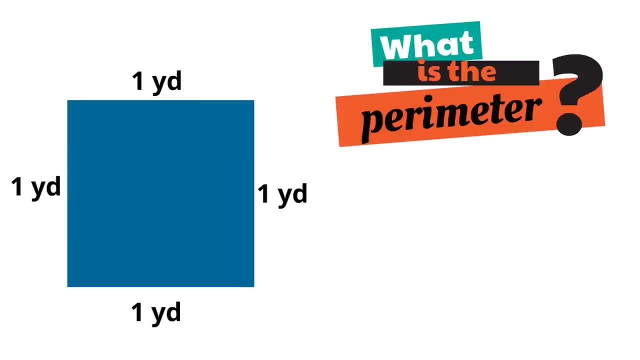 Remember, the perimeter is the distance around a shape, So we'll need to add all of these sides up. Okay, what's one plus one? plus one plus one, Yeah four. The perimeter of this square is four yards. 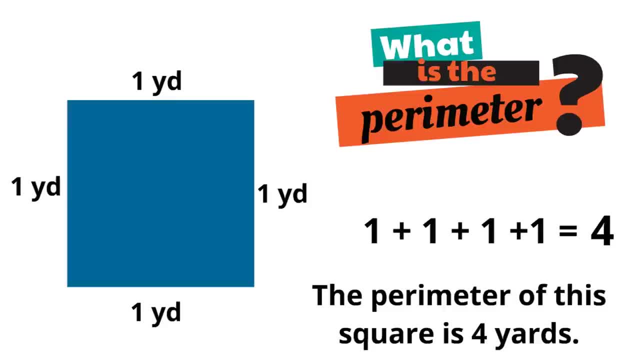 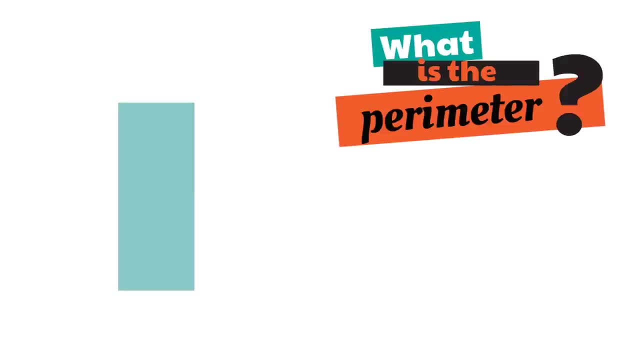 The perimeter, remember, is the distance around a shape. If you were to go around this entire square, it would be four yards. Okay, this is the final one. What is the perimeter of this rectangle? Well, first we need to know how long all the sides of the rectangle are. 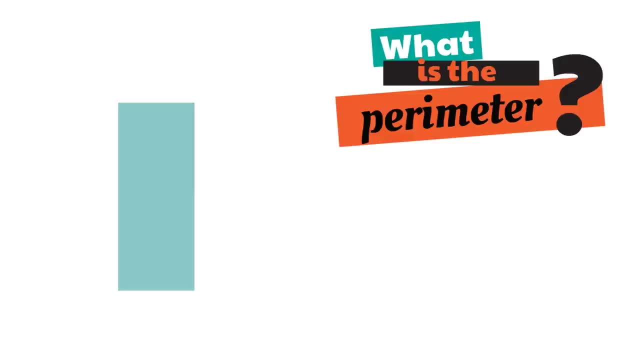 Then we can figure out the perimeter. Remember, a rectangle has four sides and two of the sides are shorter than the other two sides. With this rectangle, let's pretend we measured it at one meter on the short sides and three meters on the longer sides. 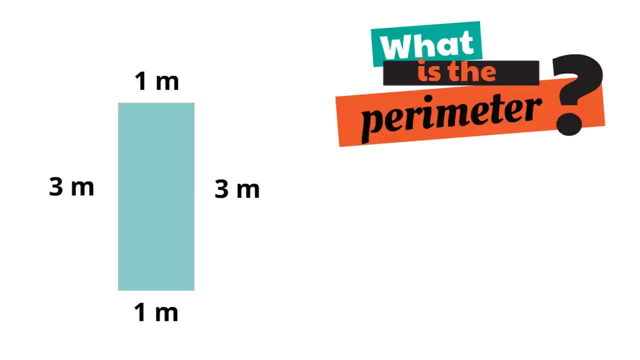 Okay, remember, to get the perimeter we have to add all of the sides together. So we're going to be adding four numbers together. again, To make it easier, we're going to group the smaller numbers together and then put the larger numbers in our equation.